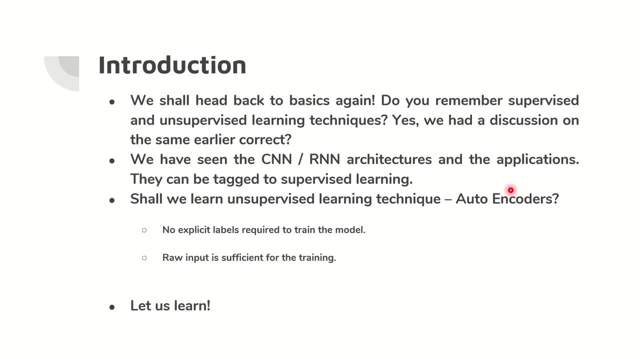 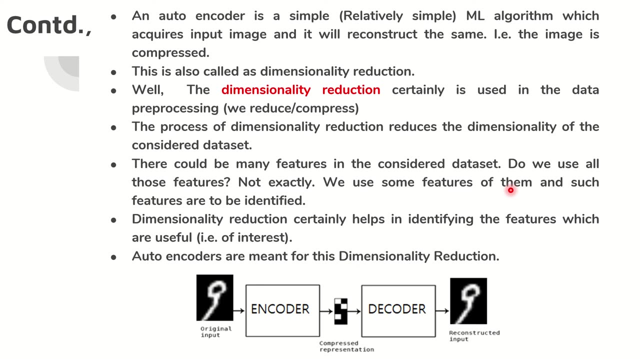 to train the model and raw input is sufficient for the training. These two points are fundamentals and remember it. No explicit labels required. raw input is sufficient for training the model. Let's get into the core area. An auto encoder is simple As compared to ML or deep learning. 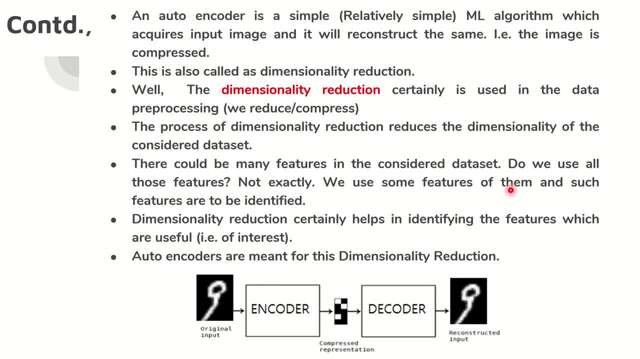 algorithms. whatever we have learned till now, it is definitely simple. It is relatively a simpler model which is going to be used for training the model, So let's get into the session. Very Clint Now. what we wish to achieve with AC is to use emailMaverick Facebook mobile email. 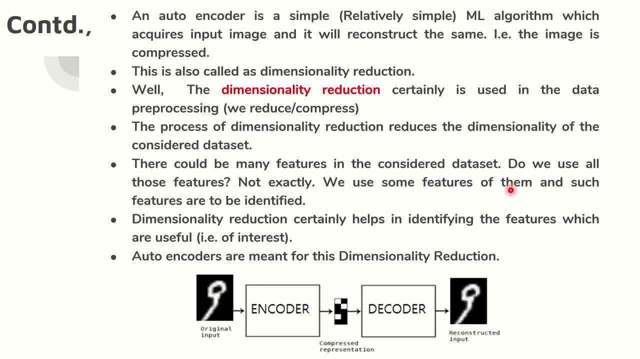 and other payment methods. The same goes for Microsoft Office, More booked and familiar for Kane, read on and off almost monthly. Ok, the next point is self development, so I hope you have understood me well. inhalation function can work and also help people grow their dataΘast times. 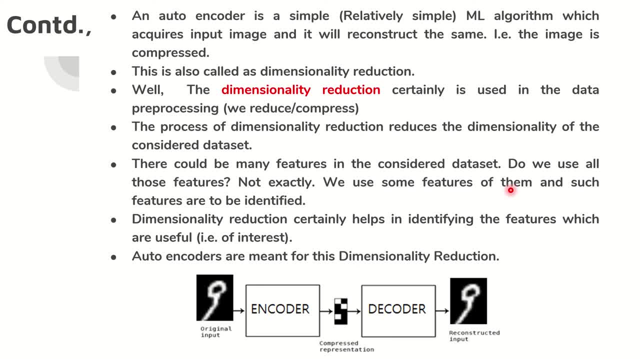 Well, I've covered this four-part theory here. Today's content is less Anglo-, иногда Jest dimensions, I mean reduce the dimensionality of the considered data set. What do you mean by this? A very simple example: when I am considering a data set or, for example, an image, there. 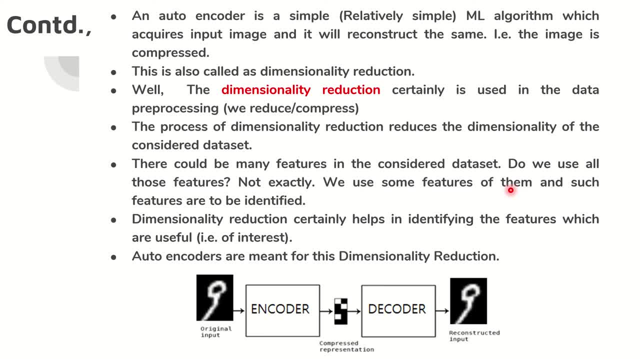 could be multiple features that are attached to it. Do I need all those features? No, I may need only few of them. So dimensionality detection will help you in acquiring only those features which are of your interest, and that's what it is all about. 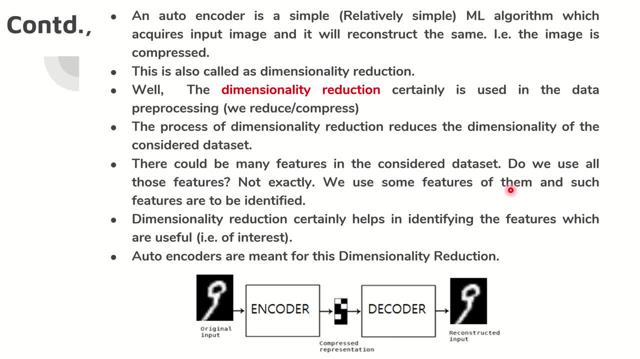 Auto encoders are 100% meant for this dimensionality detection. You can see a simple picture that I have given here. the original input is given into the encoder and the compressed representation happens here. the compression happens here and then the decoder decodes it and reconstructs the input. 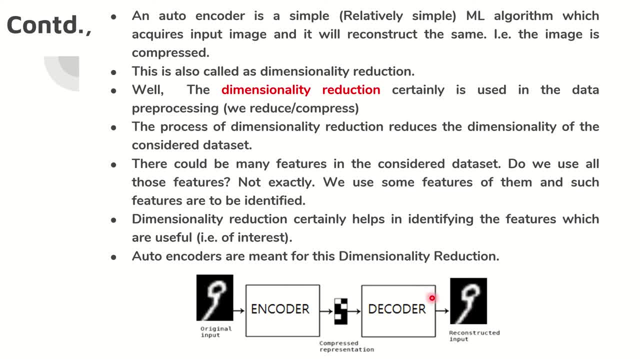 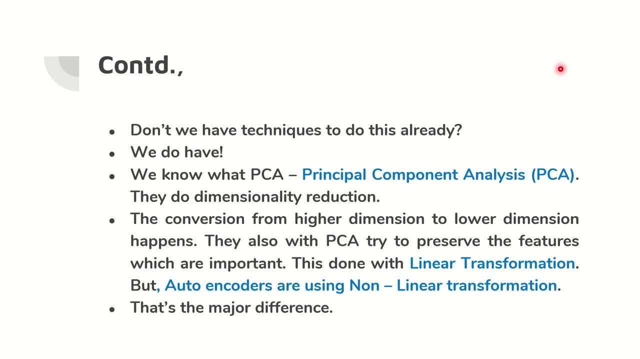 The input and output are the same. but I will have a catch for it. maybe a little later I will explain you what it is Right. don't we have any other techniques till date for this purpose? Yes, we have got few. PCA is one of them. Principal Component Analysis. 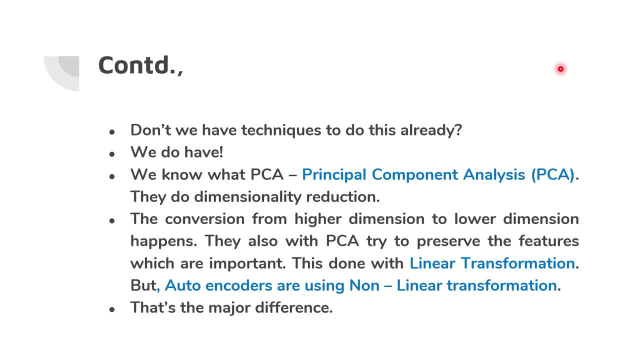 What is it? Very simple. they also do dimensionality detection, But only difference between dimensionality- I mean the dimensionality detection done by PCA and auto encoders- is the PCA will go ahead with linear transformation, whereas the auto encoder will go with non-linear transformation. 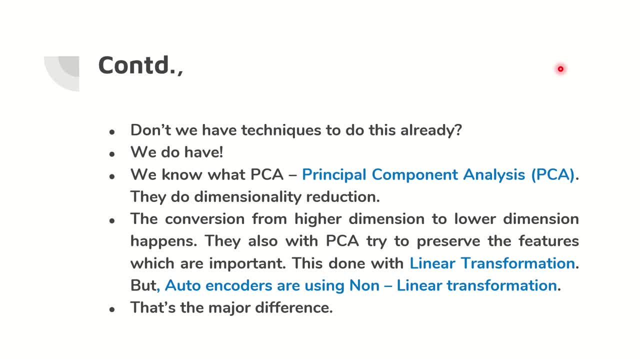 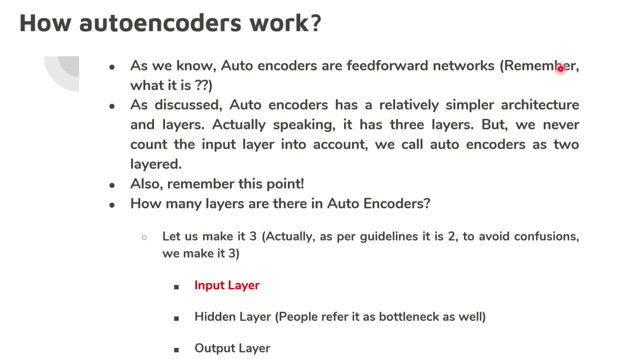 The dimensionality detection happens through linear transformation in PCA. it happens through non-linear transformation in auto encoder. that's the major difference. Right, how auto encoders work? Very simple, they are feed forward networks. I told you what is feed forward networks: from the left it goes on to the right. no, 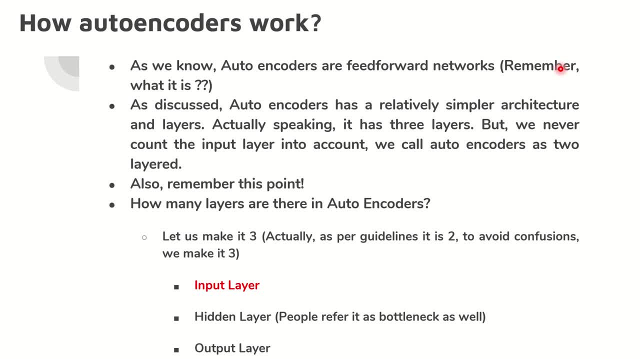 coming back, a particular point will not be reached twice. that's it. just remember that point. Right, auto encoder has got three layers: input and the intermediate layer, the final layer, the input layer, the hidden layer and the final layer. 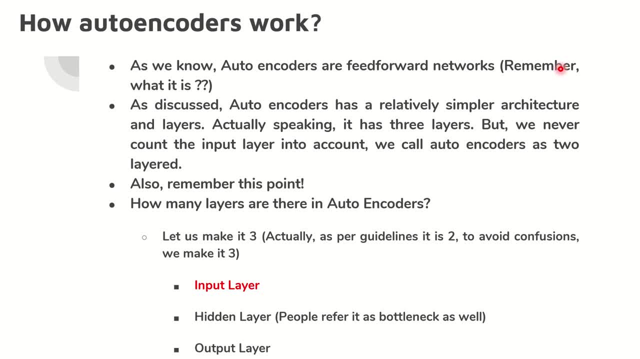 The input layer is normally never considered when you talk about neural networks, so officially it is two. We have three layers. officially it is two. Obviously it is two layers. the hidden layer and the output layer are the most seen and valued layers when you talk about neural networks. 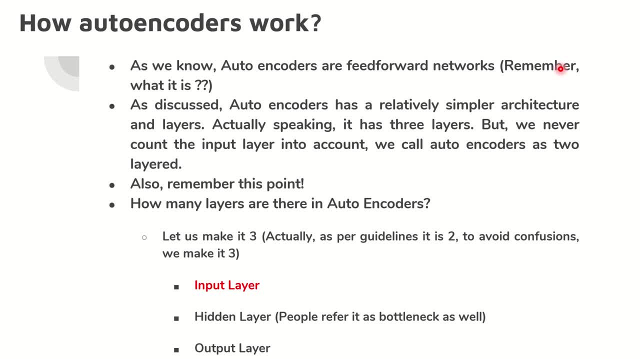 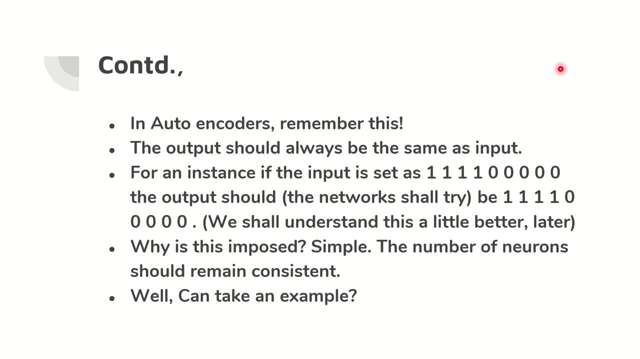 The hidden layer is also referred as bottleneck. remember it: the hidden layers are also referred as bottleneck. Now understand this final point. this is very important. again, to conclude what auto encoders are all about. I am going to give an input as 11110000 to the system, I mean to the auto encoder. 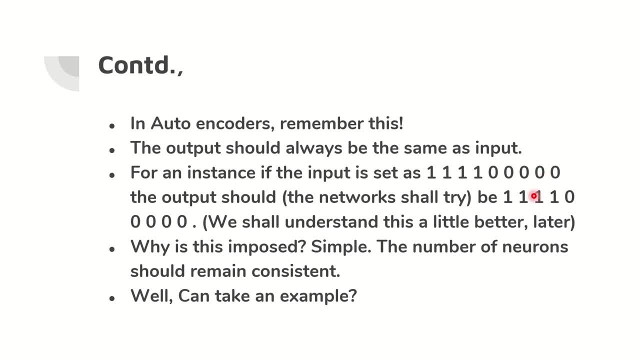 So what will happen? The system will not give input. The system will not give input. The output should exactly be the same. 11110000 is the output that I want Now. the input is the same thing that is going to come as the output. 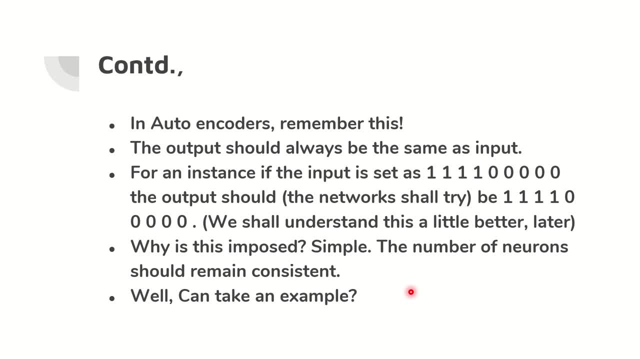 Not exactly. there is a small change or a small point that you need to remember in it. but remember, auto encoders are generally meant for just reproducing or replicating whatever input is given and the same has to be obtained as output. but there is a small catch there. 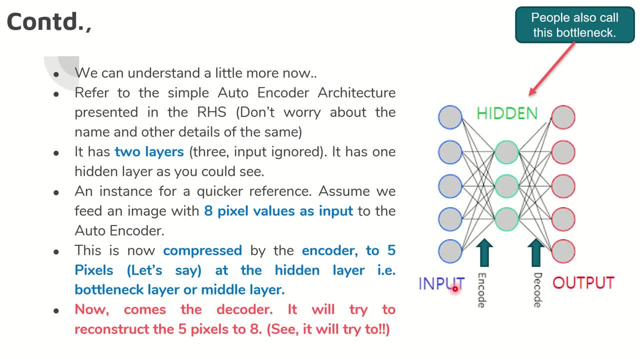 which you are going to see. I am going to present you a simple architecture of an auto encoder, which I will explain in a little later, also under a different name, and that is going to be more detailed, But for now, understand that this is the auto encoder that we are talking about. 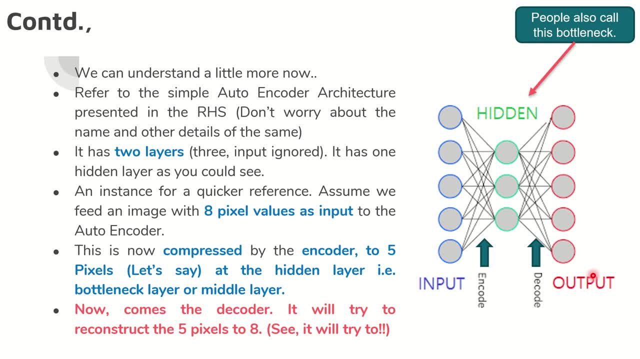 It has got an input layer, it has got a hidden layer and it has got an output layer. The input layer will send input and the hidden layer is going to do all the work for us and the output layer is going to get it. The input is encoded and before output, it will be decoded and you get the final output. 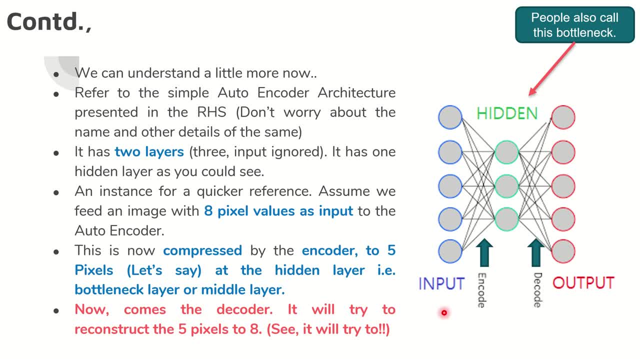 That is it. Now understand. input layer is always the same. That is it. It is always ignored when it comes to neural networks. so we are going to consider it as two layered architecture. We have got hidden layer, which is also called as bottom-net. we have got output layer and 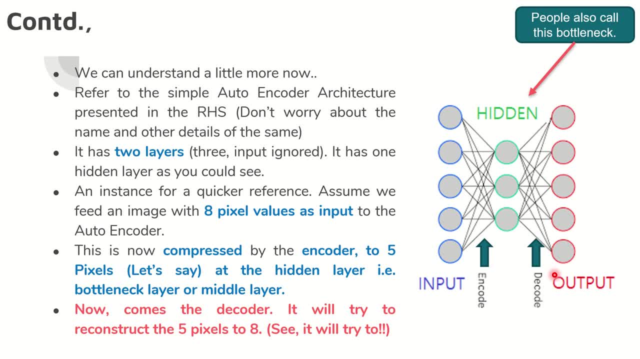 the input is encoded out here and we get it decoded and the final result Now a simple example would help you. I am sending 8 pixel values as input to this auto encoder. Now it will be compressed here as 5, for example, the 8 gets compressed as 5, but when it comes, 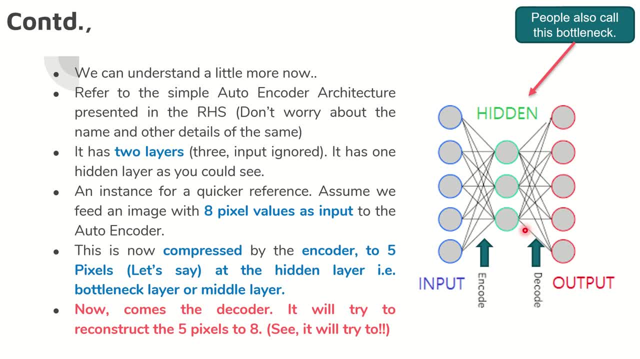 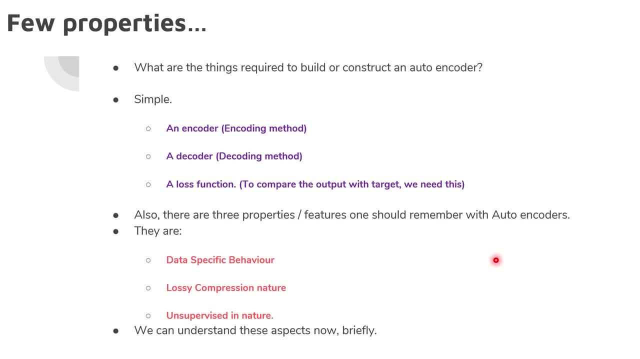 to the output layer. The reconstruction will happen and it will be reconstructed again to 8.. That is the simplest thing that you need to remember the reconstruction right. What are all the things that are required to build an auto encoder? an encoder which? 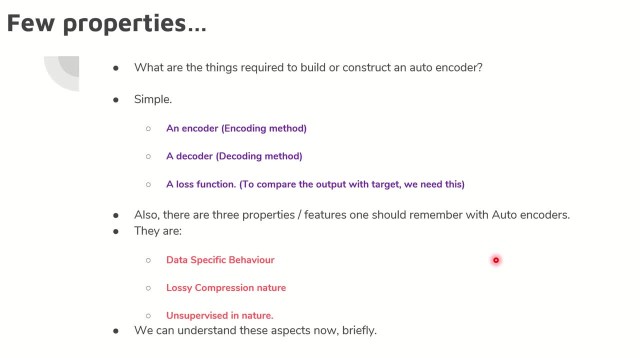 is going to do the encoding, a decoder which is going to do the decoding, and a loss function To compare the output of the target. we need this loss function and remember there are very important three features or characteristics that are normally attached or tagged to the. 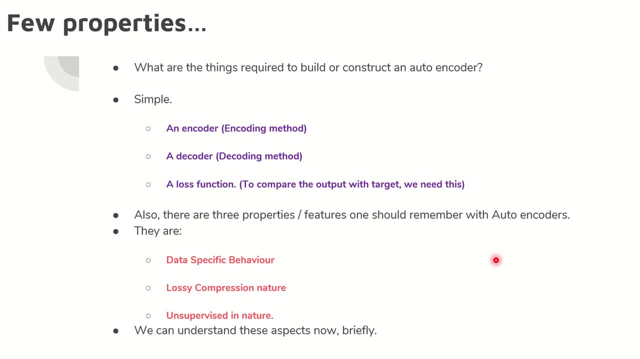 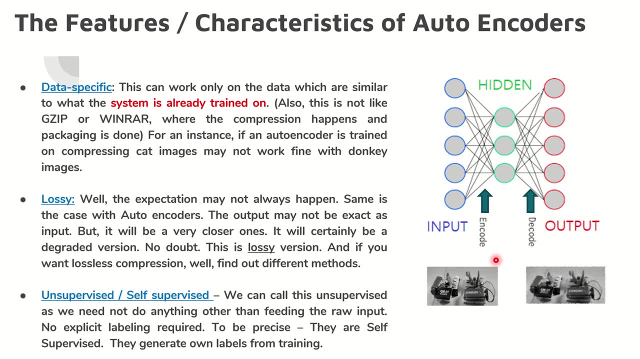 auto encoders. They are: first one, data specific behavior. second one: the lossy compression nature. third one: unsupervised nature. So what are they? We need to learn it Now. the first one: data specificity. What is this? I am training a network for specific data. for example, I am training an auto encoder. 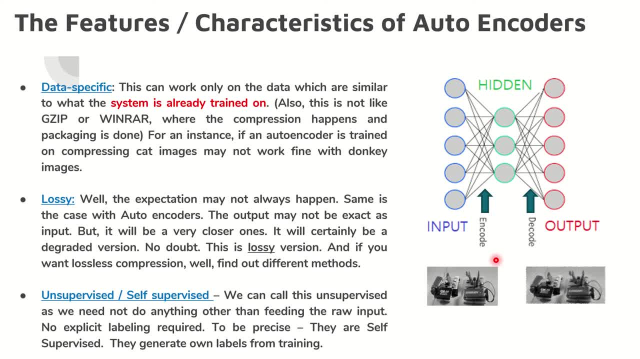 for compressing cat image. If you send donkey images, it would not understand and the results will not be as you expect. So this is working on what you have already trained on. That is called data specificity. Second: lossy: What do you mean by lossy? 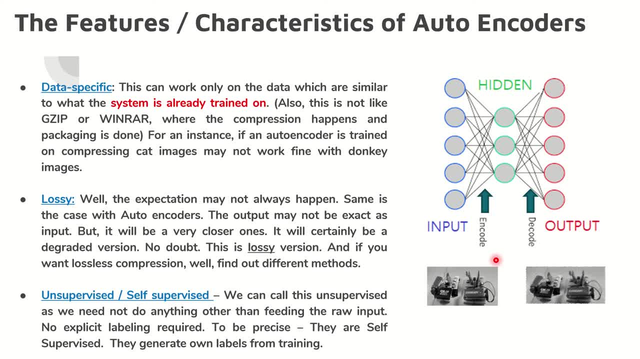 Very simple: The expectations may not be met always. What do you mean by that? I am sending an input. the output has to be exactly coming as input, but it may not happen always and there would be some loss, and this is called lossy version. 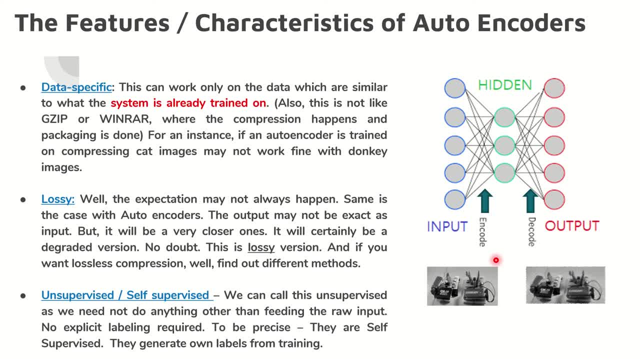 If you want no loss at all, do not come to auto encoders. it is not your option. Now next, What is unsupervised and self-supervised? It can be called unsupervised or self-supervised character. What is it?